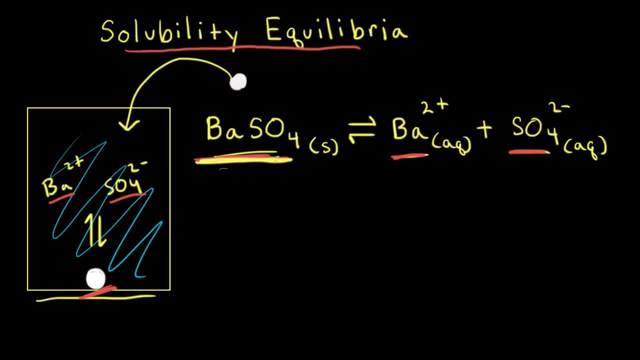 shows the dissolution of a salt, barium sulfate, And from the balanced equation we can write an equilibrium constant expression. So we would write: the equilibrium constant K is equal to the concentration of barium 2 plus, And since there's a coefficient of 1 in the 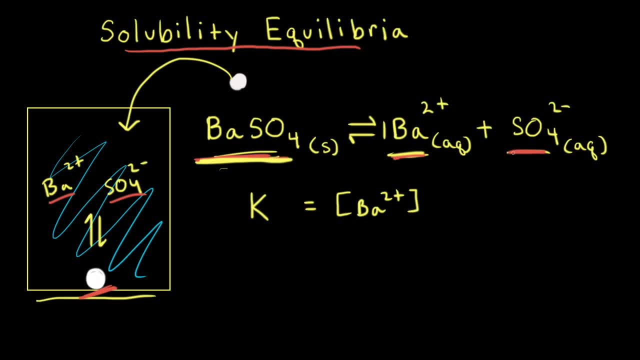 balanced equation we can write: the equilibrium constant K is equal to the concentration of barium, 2 plus It would be the concentration raised to the first power times, the concentration of sulfate also raised to the first power. And since pure solids are left out of equilibrium constant. 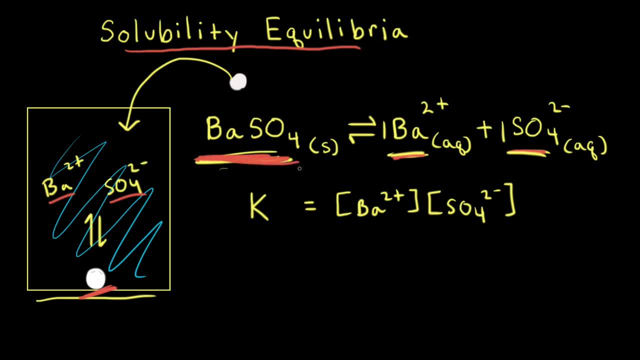 expressions. we would not include the solid barium sulfate For solubility equilibria. we would write Ksp where sp stands for solubility product, The solubility product constant. Ksp has only one value for a given salt at a constant, So we would write Ksp where sp stands for. 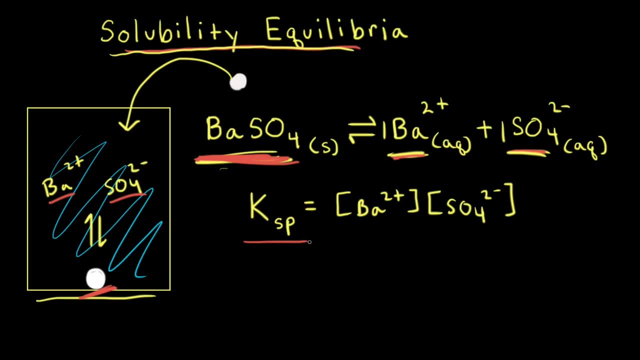 salt at a specific temperature. That temperature is usually 25 degrees Celsius, And Ksp indicates how much of that salt will dissolve. For example, at 25 degrees Celsius, the Ksp value for barium sulfate is 1.1 times 10 to the negative 10th. When the Ksp value is much less than 1, that indicates 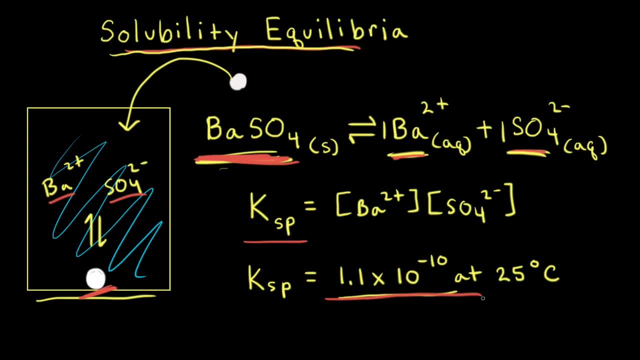 the salt is not very soluble. So barium sulfate is not a soluble salt. If the Ksp value is greater than 1, like it is for something like barium sulfate, we would write Ksp, where sp stands for sodium chloride. That indicates a soluble salt that dissolves easily in water. The solubility of a 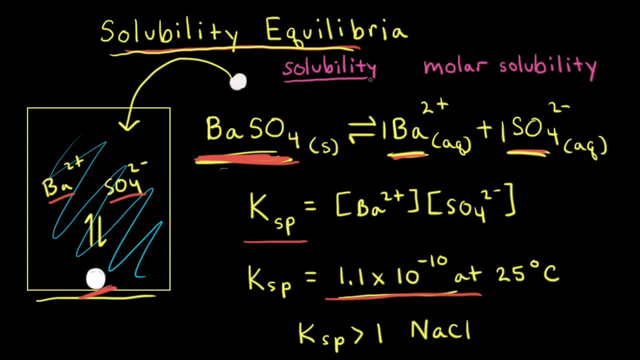 substance refers to the amount of solid that dissolves to form a saturated solution. Usually, the units for solubility are in grams per liter. Molar solubility refers to the number of moles of the solid that dissolve to form 1 liter of the saturated solution, And therefore the units would 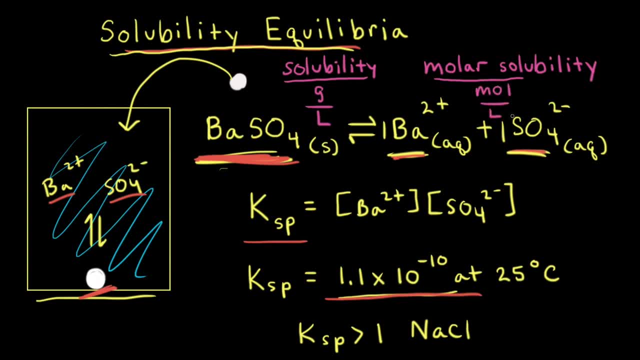 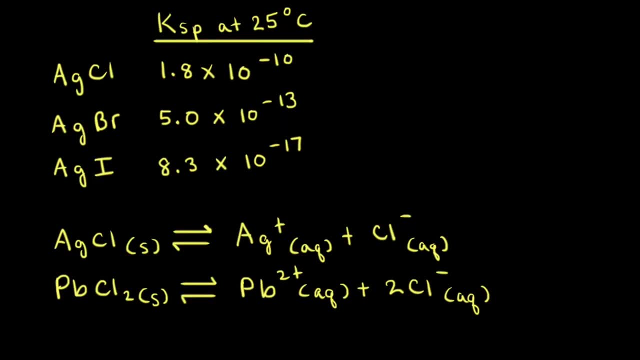 be moles per 1 liter, Or you could just write molar. Ksp values can be used to predict the relative solubilities of salts that produce the same number of ions in solution. For example, silver chloride, silver bromide and silver iodide all produce two. 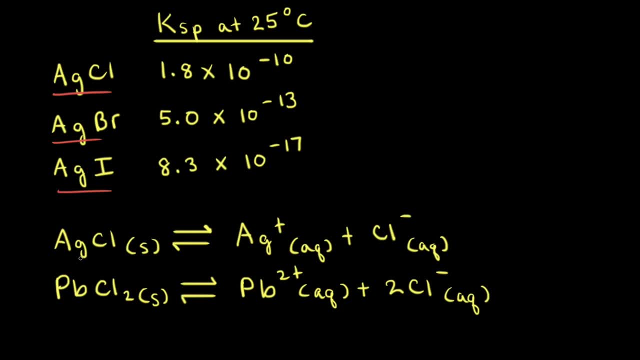 ions in solution. Let's look at the dissolution equation for silver chloride to see why this is true. Solid silver chloride turns into Ag plus and Cl minus, So that's one Ag plus ion and one Cl minus ion For a total of two ions in solution. And we could write out similar equations for silver bromide and silver iodide. 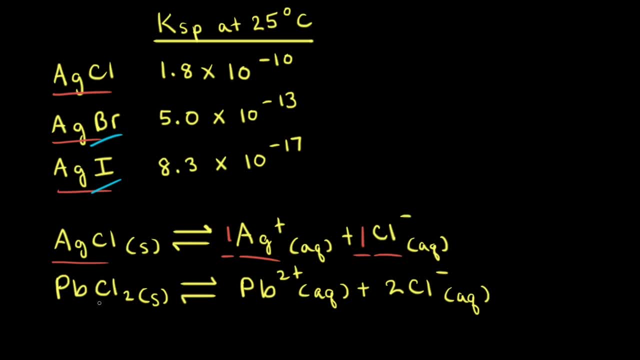 So they all produce two ions in solution. However, a salt like lead chloride produces three ions in solution. So lead chloride would give one Pb2 plus ion and two chloride anions in solution. One plus two is three ions. Since lead chloride produces three ions in solution, we can't determine its solubility relative to the other three by the 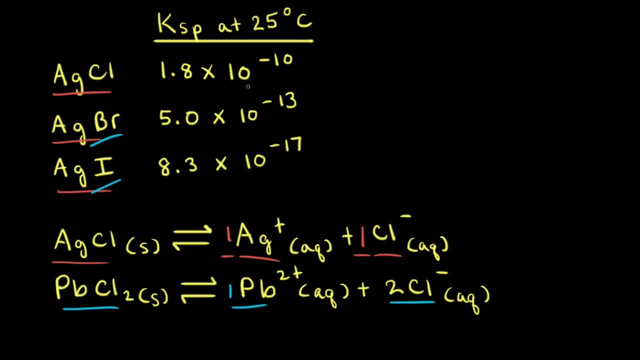 comparing Ksp values. Here are the Ksp values for the three salts at 25 degrees Celsius: For silver chloride it's 1.8 times 10 to the negative 10th. For silver bromide it's 5.0 times 10 to the negative 13th. And for silver iodide it's 8.3 times 10 to the negative 17th. 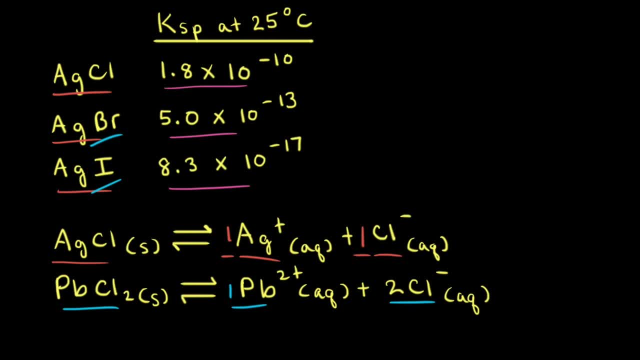 When comparing salts that produce the same number of ions, the higher the value of Ksp, the higher the solubility of the salt. And since silver chloride has the highest Ksp value of these three, silver chloride is the most soluble salt. 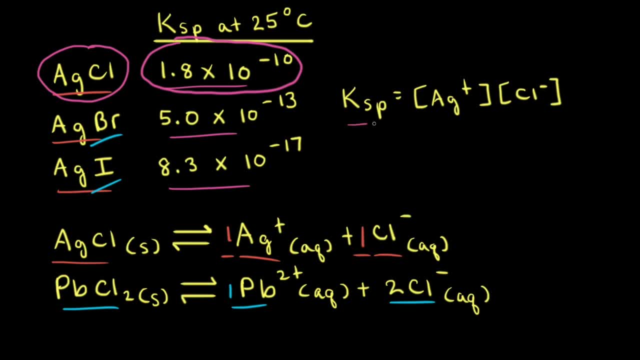 For some insight into why this is true, let's look at the Ksp expression for silver chloride, which we can get from the balanced equation. The higher the value for Ksp, the higher the concentration of these ions at equilibrium, which means that more of the solid must have dissolved. 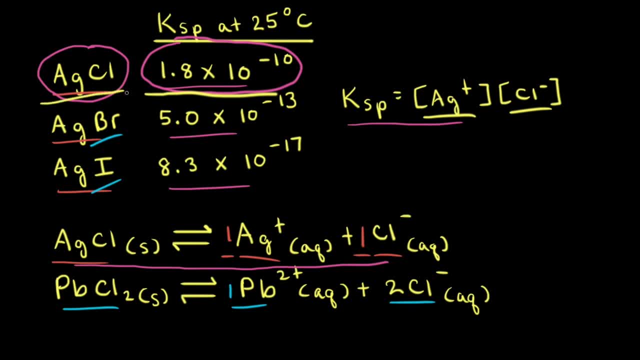 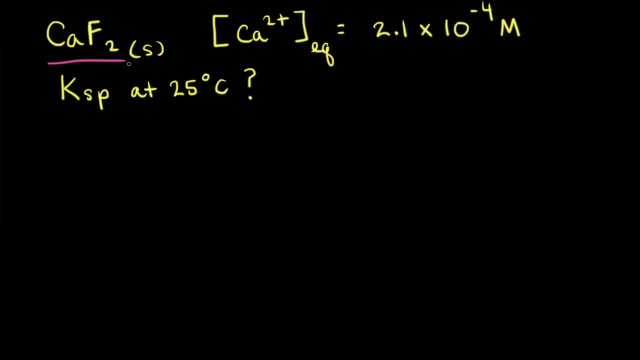 Therefore silver chloride has the highest solubility out of these three salts. Let's say we have some solid calcium fluoride that we add to pure water at 25 degrees Celsius. Eventually equilibrium is reached and the equilibrium concentration of calcium two plus ions. 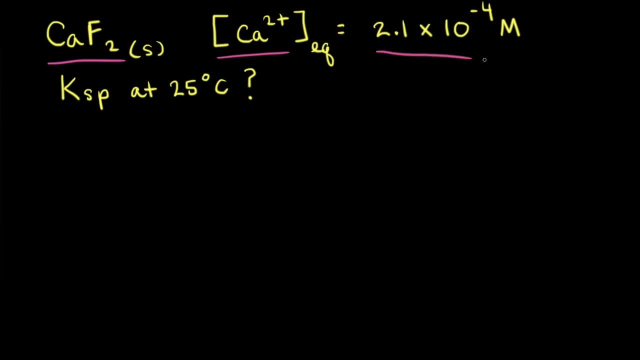 is measured to be 2.1 times 10 to the negative fourth molar. Our goal is to calculate the Ksp for calcium fluoride at 25 degrees Celsius. The first step is to write out the dissolution equation for calcium fluoride. So we would write: CaF2 solid. 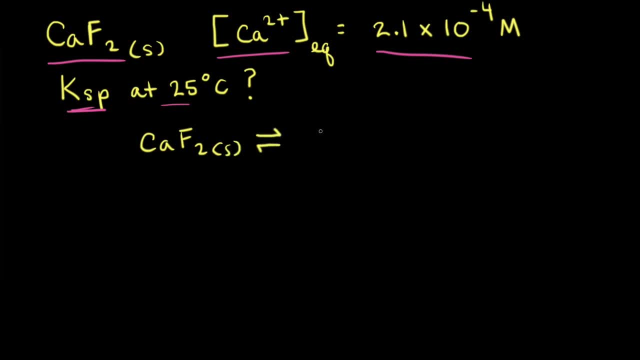 and we know that calcium forms a two plus cation. So we would write Ca2 plus an aqueous solution, And to balance everything we'd need two fluoride anions, So two F minus also an aqueous solution. The next step is to use the balanced equation. 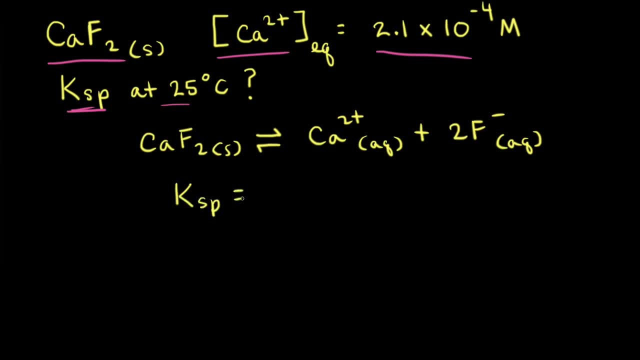 to write the Ksp expression. So Ksp is equal to: there's a one as a coefficient in front of Ca2 plus. so it'd be the concentration of Ca2 plus raised to the first power and then calcium overlapped to ди abuse. 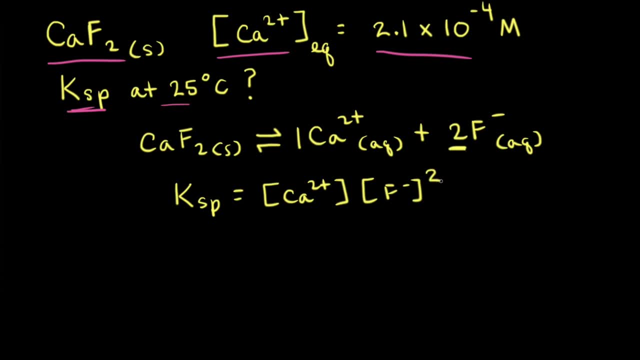 in翻 swoop. two to three, including calcium fluoride. Here's the concentration of calcium fluoride being re lineup Red over three and it'sбаgasо. this is the concentration of fluoride anion and since there's a, two is a coefficient. 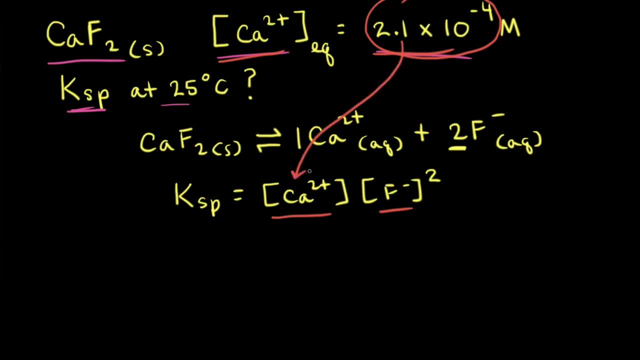 this is the concentration of fluoride an ion squared For a Ksp expression. these are equilibrium concentrations and we already know that the concentration of calcium two plus that equilibrium, we need to plug in the equilibrium concentration of fluoride anion. Well, looking at the dissolution equation, 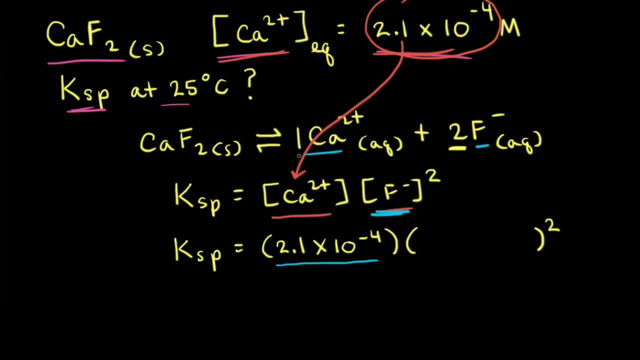 the mole ratio of calcium two plus to fluoride anion is one to two. Therefore, at equilibrium there's twice as many fluoride ions in solution as there are calcium two plus ions. Therefore the equilibrium concentration of the fluoride anion would just be twice this concentration for Ca2 plus. 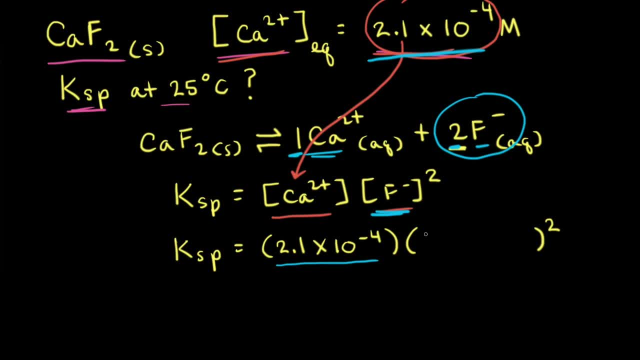 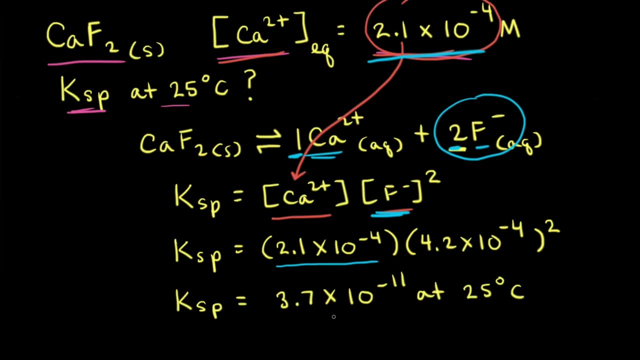 So the equilibrium concentration of fluoride anion must be 4.2 times 10 to the negative fourth molar. And when you do the math you get that Ksp for calcium fluoride is equal to 3.7 times 10 to the negative 11th. 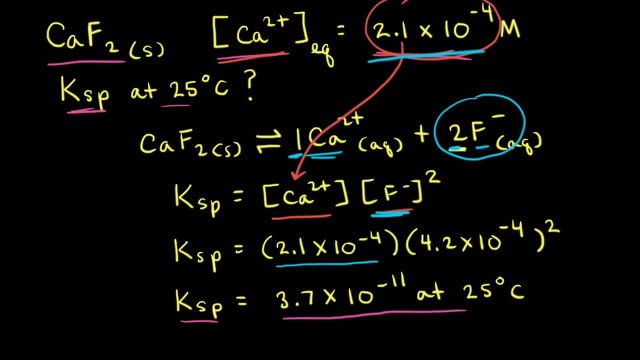 at 25 degrees Celsius. Ksp values can be difficult to measure and therefore different sources often give different values for Ksp at the same temperature. For example, for calcium fluoride at 25 degrees Celsius, one source had Ksp equal to 3.5. 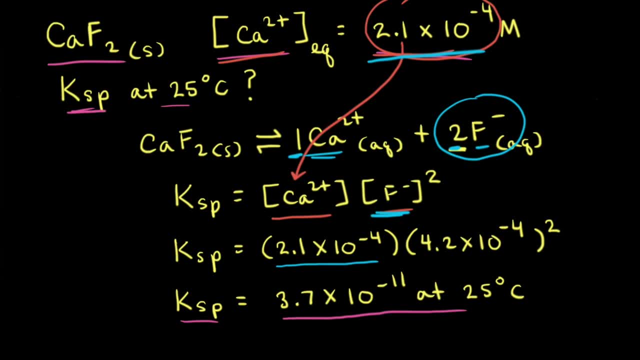 times 10 to the negative 11th. Another one had 3.9 times 10 to the negative 11th. Since we got 3.7 times 10 to the negative 11th, this sounds like a pretty good calculation. 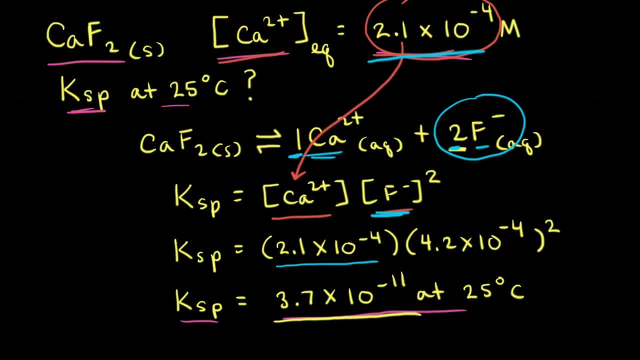 for the numbers that we used for our problem. Finally, let's think about the molar solubility of calcium fluoride. So how many moles of our salt dissolve to form one liter of our saturated solution? Well, the mole ratio of calcium two plus ions.